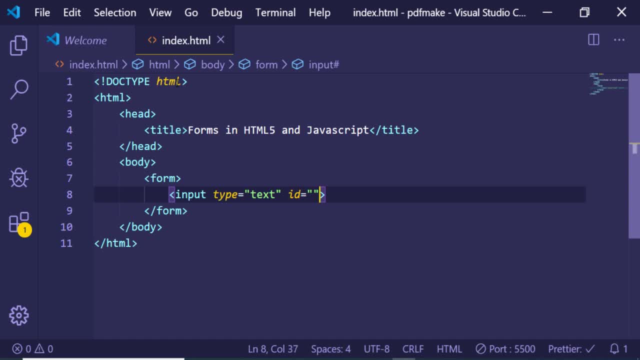 text we will be having- let me just give it a simple ID of username, and also we will be having another field input type of email. here we will be submitting our email, so ID will be email and you can even have a validation also required. so this is html5 validation. 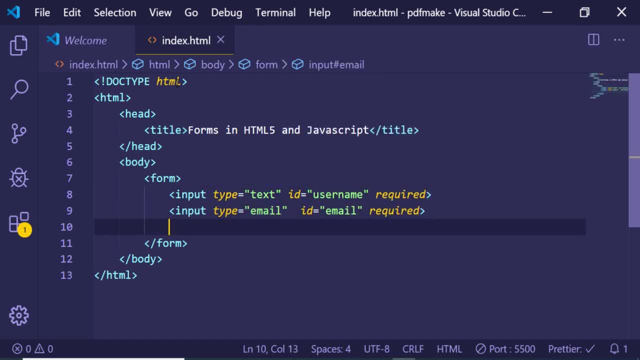 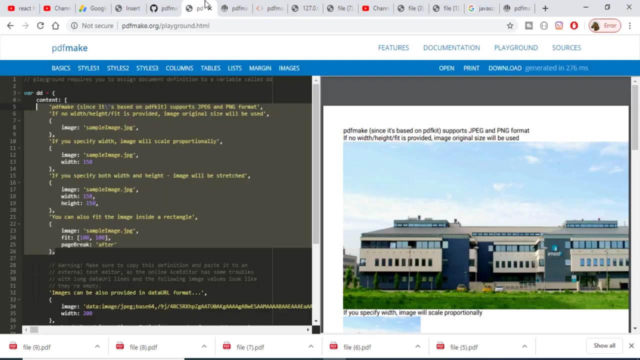 rule. so you should enter this value, so it is required. and lastly, we will be having a button- so input type, submit, which will submitting our form. so let's suppose I have register and now, if I just refresh it, my application, you will see that a form will be constructed. let me just move on to me refresh the you. 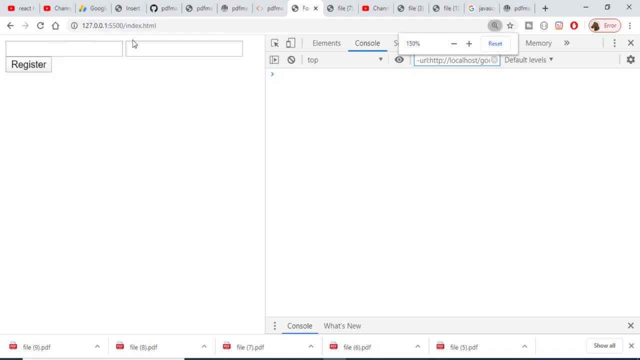 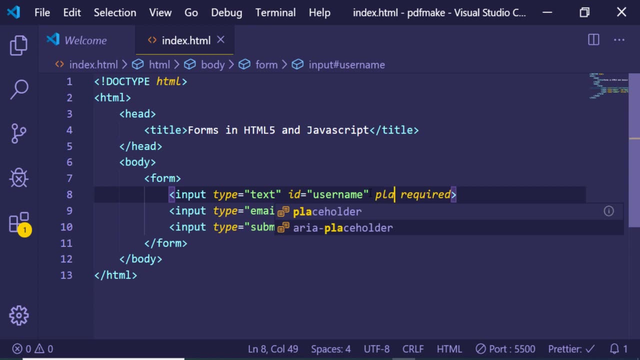 can see that two input fields are there. let me just zoom in. first is the username and second is the email and register is there. so if you have to add a placeholder, you can even add a placeholder. let's suppose it is username, just to add a hint to the user, and placeholder is email, like this: and now: 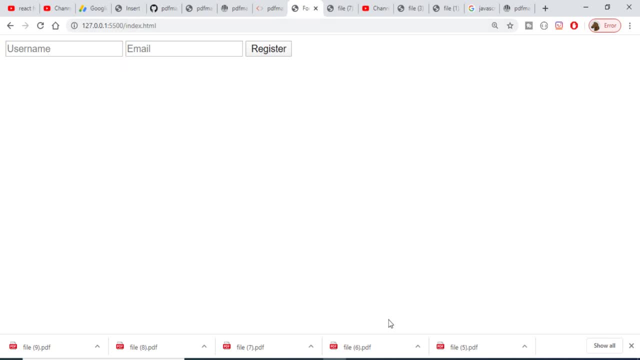 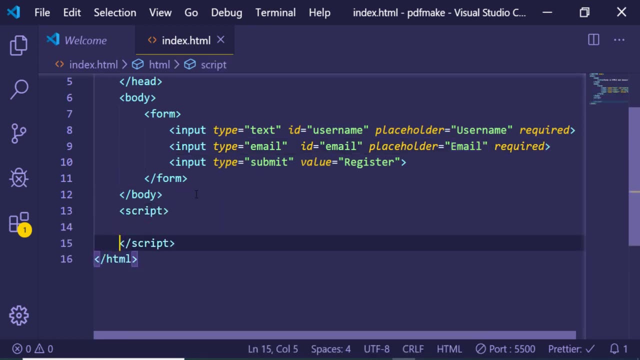 again. if I refresh it, you will see the placeholder which is coming here and now we just need to write our JavaScript code in order to handle this form. so just have a script tag and inside this form, we will be having a placeholder. so this, first of all, in order to get the reference to the form you will be giving. 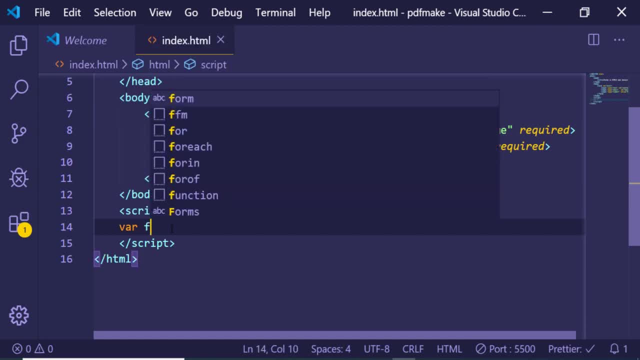 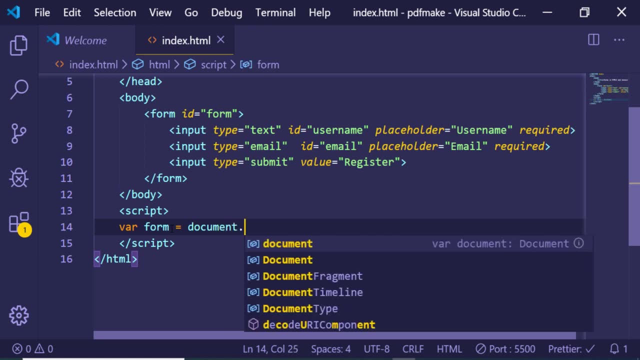 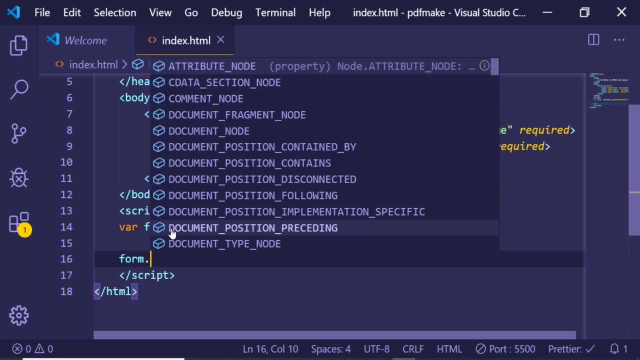 an ID to it of form like this. and now, in order to get the reference, we will be invoking a very simple method, which will be get element by ID on the document variable, get element by ID, and here we will be passing the ID that we have given to the form, which is form. and now the second step is: guys, we need to add: 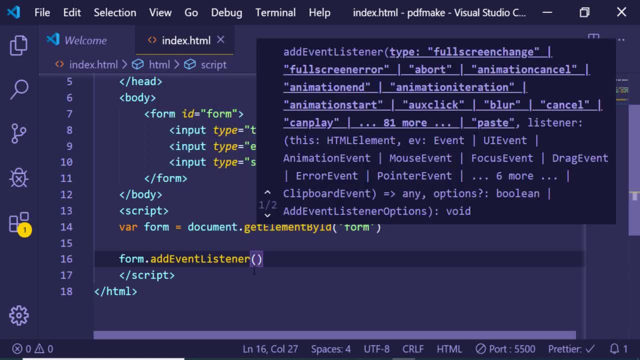 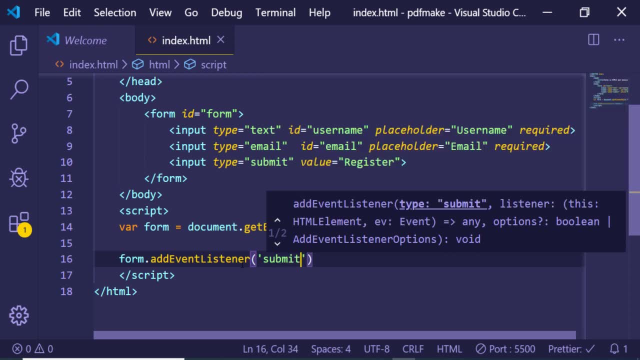 event less listener. so basically, event listener in JavaScript is something that whatever event happens. so there are various events out there in JavaScript. first one of them is submit. so when the form submits, this callback function will execute. it will hold the event object. so this event or object automatically get. 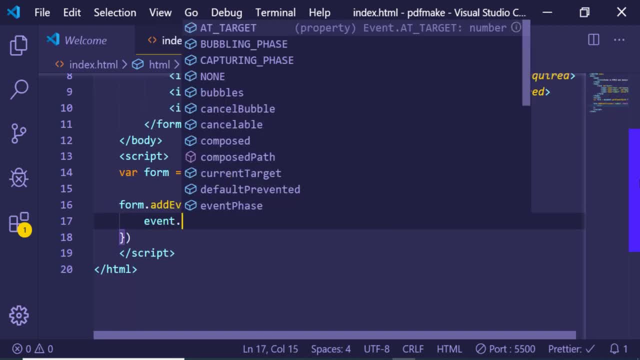 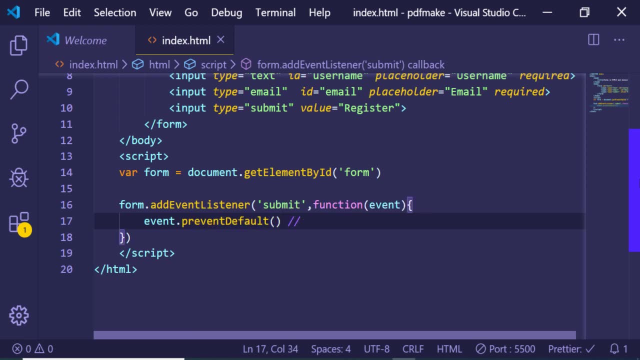 passed whenever the form submits. and now, inside this event object, there is some methods that you can pass, which is event prevent, default. so basically, let me write a comment and explicitly explain to you why we are doing this. basically it is it prevents the form from auto submitting. so what do you mean by auto? 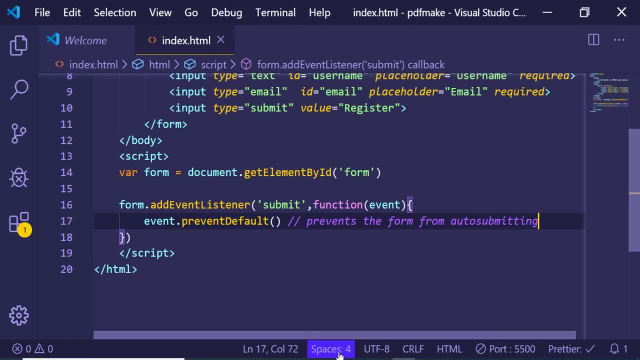 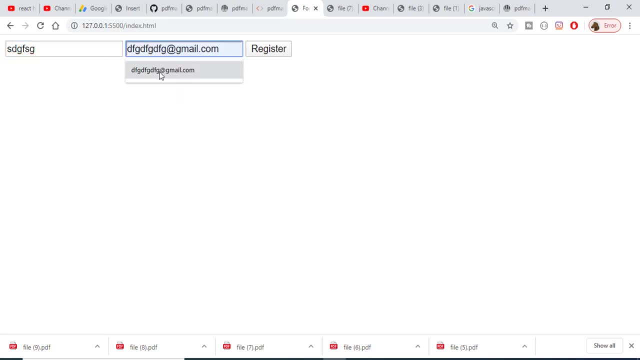 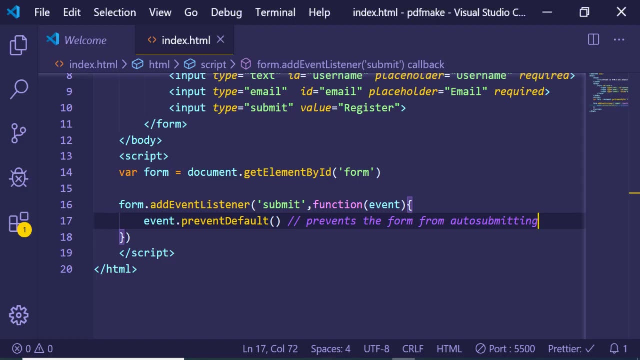 submitting. auto submitting basically. basically means that whenever we make a form, we enter values here: username, and let's suppose I enter an email address and click on the register button now, the now it will auto submit. so with the, if I just uncomment this line here, if I don't write this line, you will see a question. 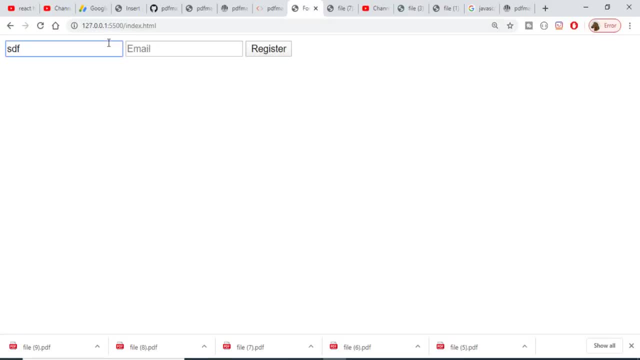 mark appearing here right now. I have to do something right now, so I have to do right here in inside the browser. so if you, if I see you, if I write the email address and click on the register button, you will see the question mark. so it is auto submitting. so now it is not. 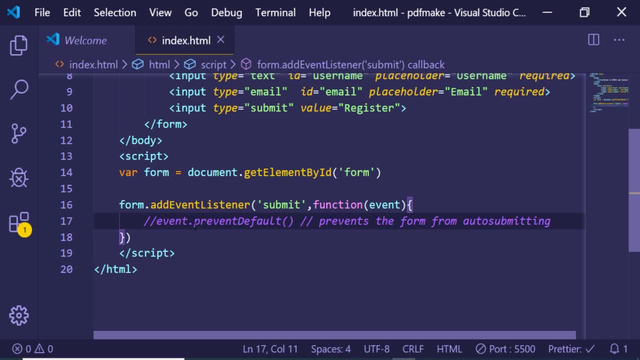 processing my code which I have written inside this form, even add event listener. so that is why I am just invoking this method, so that it will auto prevent the auto submitting of the form. so it is a very important line that you need to write so now. after that we can just grab the values that 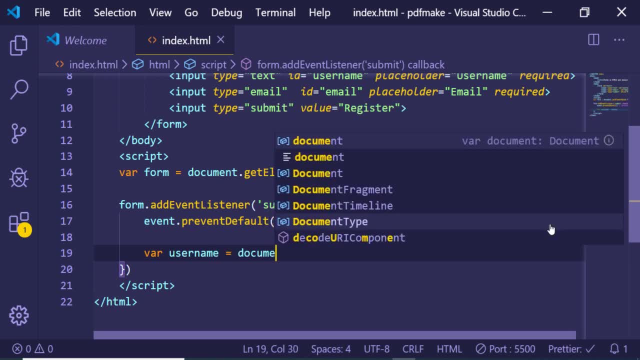 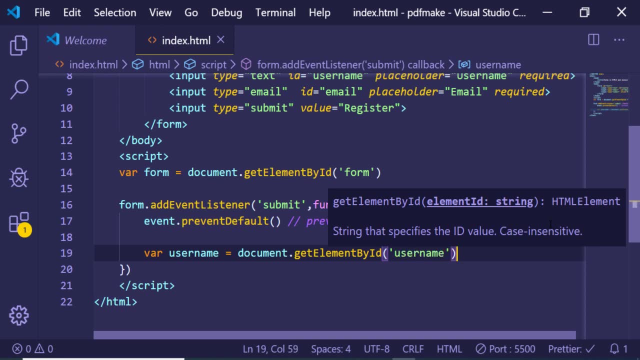 the user has typed first is the user name. so again we can just follow the same formula. we can just get element by ID, and this time we have given the user name, the ID of user name, and after that we need to dot value. so this will extract the value that the user has typed inside the user name. 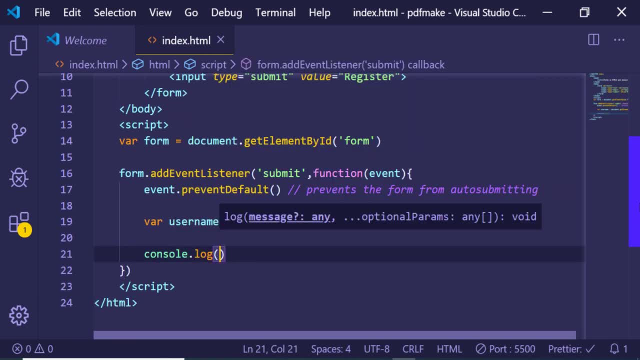 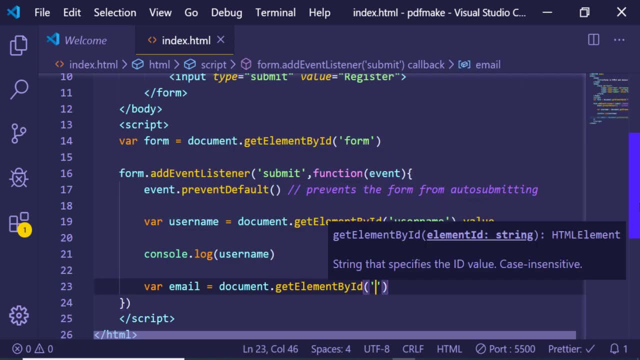 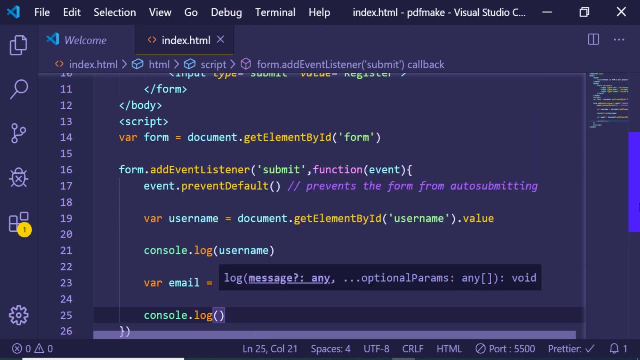 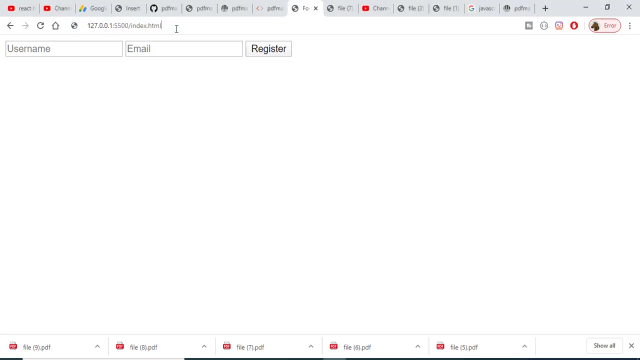 field we can console of the value, also to cross check user name. and now the second field is email. so email. we will be following the same formula. we will supply email dot value. so this will grab the email address, and now we can console log also this email address. so now let me just show to you what I mean by that, in order to see the console log. 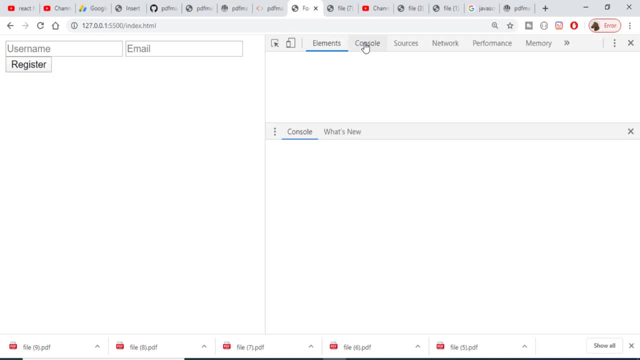 messages. you need to right click, go to inspect and go to console. so here, all over the console log messages will be printed out. so let me write an email address. click on register. you will see that both the things have printed out in the console. log messages will be printed out in the 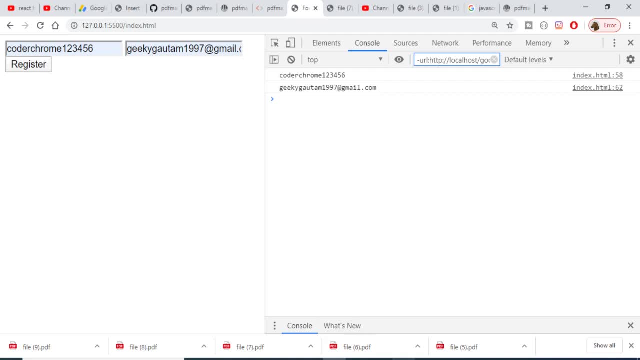 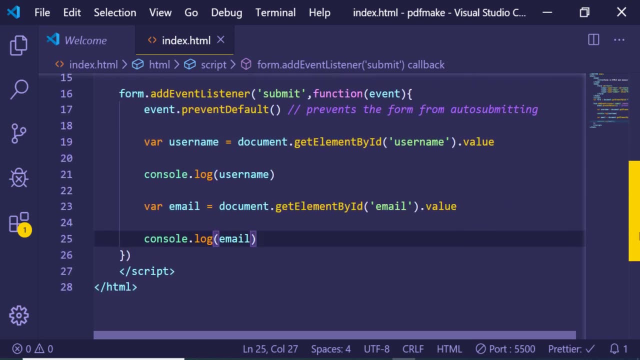 console successfully, username, email address, and now you can just process this form and do whatever that you want to do: make a get request, just store it inside your database. so basically, this is the step-by-step formula in order to process forms in any kind of application that you are making.